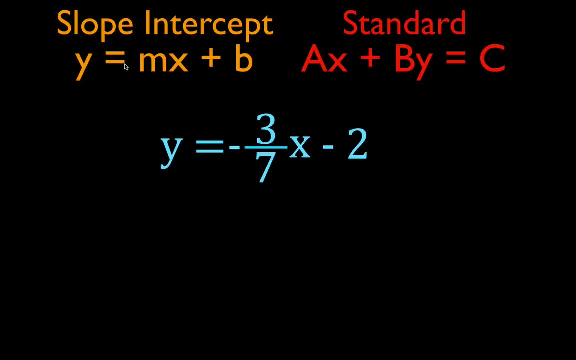 form, which is: this is the general form for the slope-intercept form: y equals mx plus b. You'll see we have y equals minus 3 sevenths. Minus 3 sevenths is the slope, m stands for the slope. b is the y-intercept. We have minus 2 as our y-intercept. Y equals mx plus b. 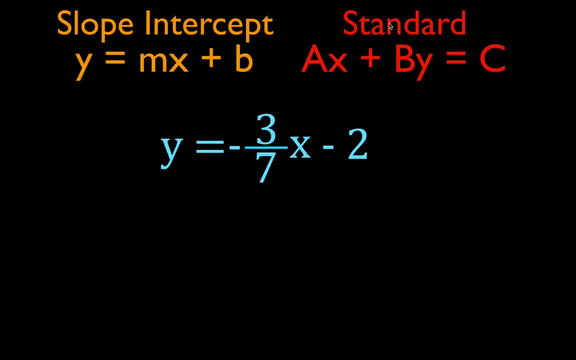 the slope and the y-intercept. This is the standard form. This is the general form of the standard form ax plus by equals c. We want to convert this from the slope-intercept form to the standard form. In the standard form, a and b, the coefficients must not be fractions. They 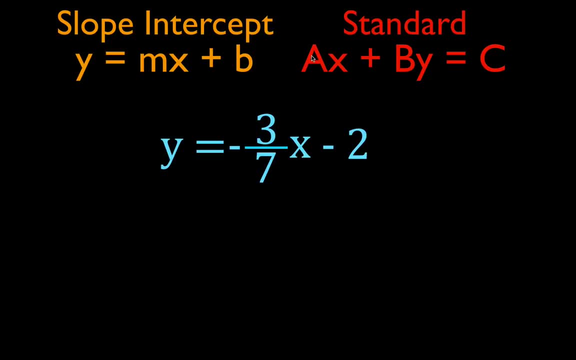 cannot be fractions, And a, the coefficient a, should be a positive number. We've got to make sure we take care of all those things. Now you'll notice in the slope-intercept form, everything is on the right-hand side except for the y. Everything is on the right-hand side except 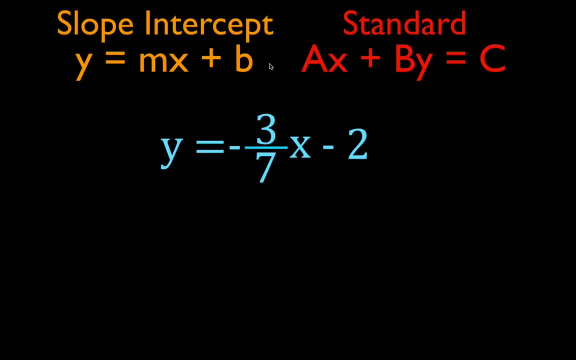 for the y. In the standard form, everything is on the left-hand side except for this final integer, So we need to basically move the x term to the other side. The y is already on the left-hand side. We've got to get the x term to the other side and clean it all up, so we have no negatives. 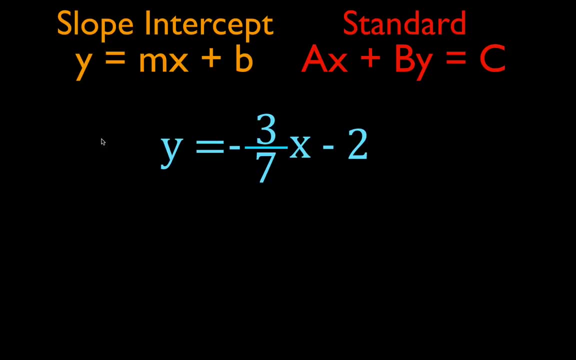 And no fractions. Now there's a couple ways you can start. I like to start like this. Step one: if the slope now m in the slope-intercept form, m is the slope, the number in front of the x. Well, the number in front of the x is a fraction. So if the slope is a fraction, in this case the 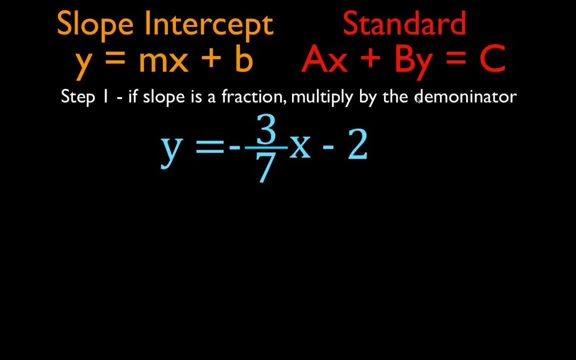 slope is minus three-sevenths multiply by the denominator. Basically, we want to get rid of the fraction, So we're going to multiply the whole equation By the denominator. the denominator is seven. multiply it by seven. I'm going to distribute. 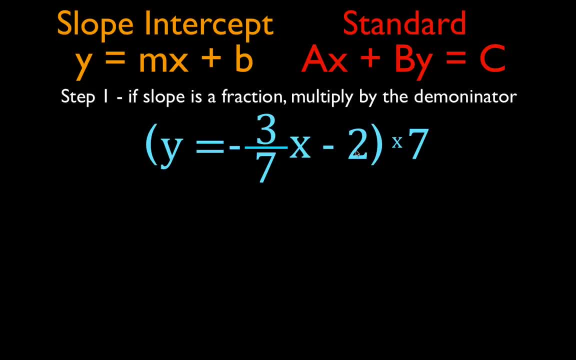 seven through these three terms: one, two and three. Seven times y is seven y. Bring the equal sign down: Minus three-sevenths, x times seven, the sevens cancel and you're left with minus three x. Minus two times seven is minus fourteen. That is step one. We multiply it by the denominator. 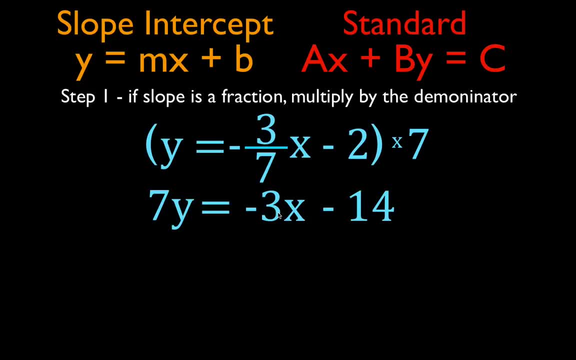 we got rid of the fraction and therefore that's the end of step one. Step two: now we're going to add the opposite of the x term to both sides of the equation. The x term is minus three x. Well, the opposite of minus three x is three x. I'm going to add three x to both sides. Here's my. 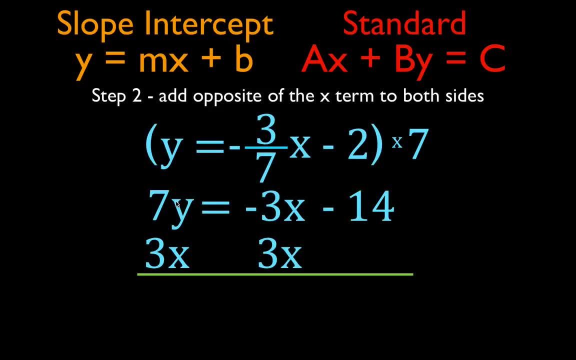 equal sign: the left side, the right side, Seven y plus three x. It's not like ten x y or twenty one x y. We're adding. These are not like terms. This is like apples and oranges: You can't add. 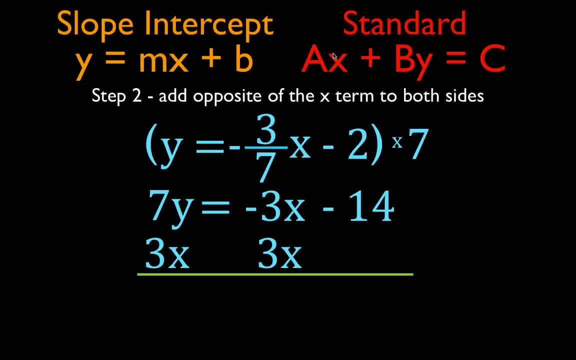 apples and oranges. We have y and x, So we put the x term first and then the y, so we're just going to write down three x plus seven, y, A x plus b, y, A x plus b- y. Bring the equal sign down Now. 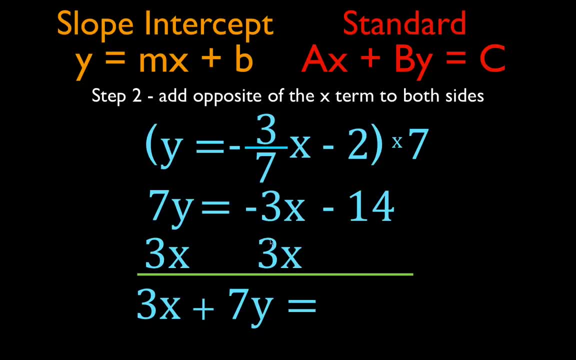 we have minus three x and three x. When we add minus three x and three x, we get zero. So people say they cancel, and then you just bring down the 14th or the minus 14th. That is the. that is that. 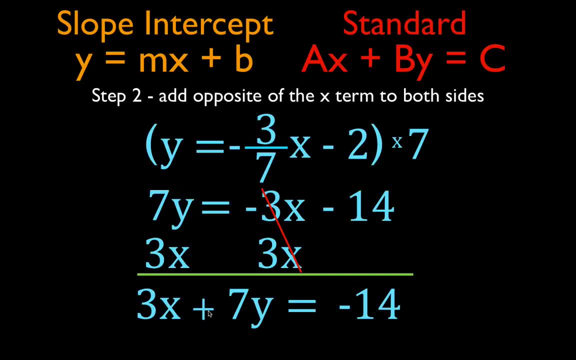 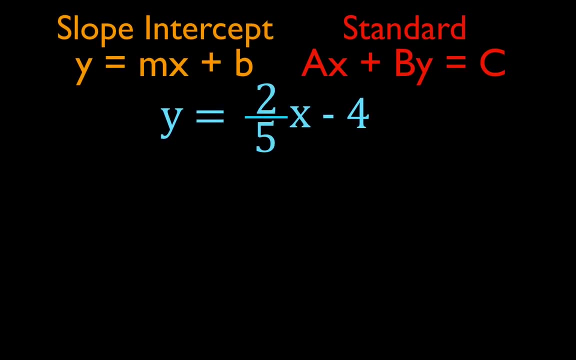 equation in the standard form: A, x plus b, y equals c, No fractions. The a term, the coefficient a is positive and there we go. Next one: We're going to do the same two steps. Step one was: if the slope 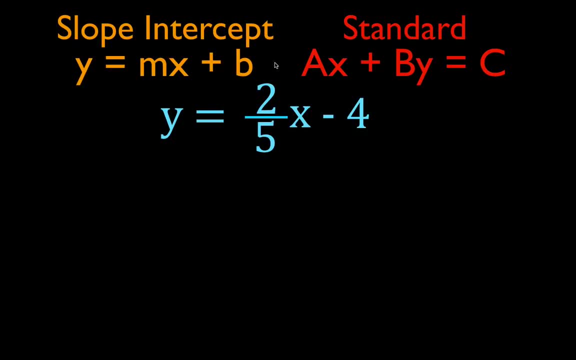 the number in front of the x term was equal to zero. So we're going to do the same two steps. So the x is the slope mx, If the slope is a fraction, multiply by the denominator. So you can see: two-fifths is a fraction, the denominator is five Multiply by five. So I'm going to distribute the 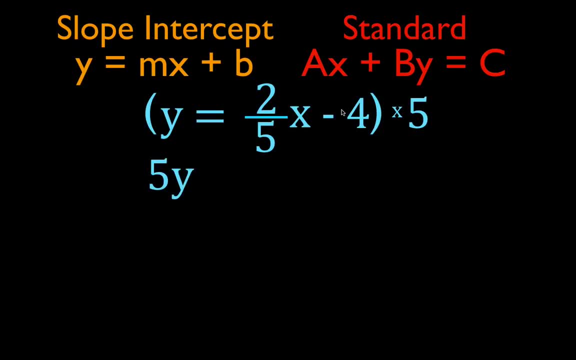 five through all three terms in this equation. Five times y, five y Equal sign. Two-fifths, x times five, The fives cancel. You just get two x minus 4 times 5 is minus 20.. That's step one. 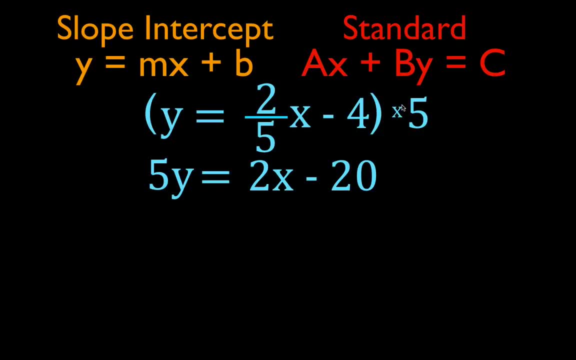 Multiply by the denominator of the fraction, if the slope is a fraction. Now the second step is to add the opposite of the x term to both sides. This is 2x. the opposite of 2x is minus 2x. so I'm going to write down: 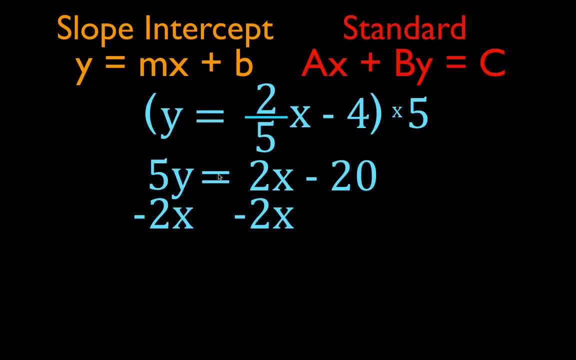 minus 2x and minus 2x on both sides. Once again, y and x, those are unlike terms, those are not like terms, And it's ax plus by. so I'm going to put down minus 2x plus 5y. 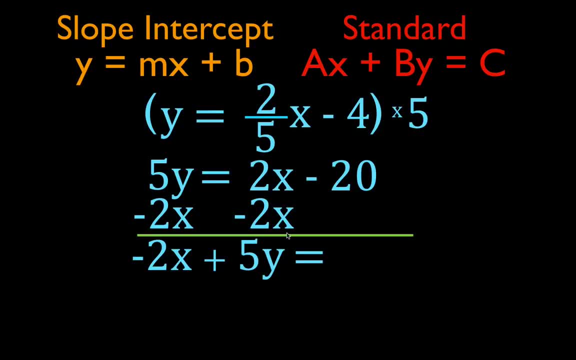 We have plus 2x and minus 2x and we add those, we get 0. They cancel and therefore you get minus 20.. Now you can see we're almost there. We did say that in the standard form the x term may not be negative. 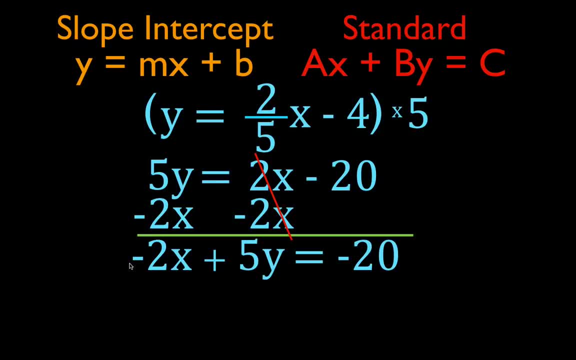 Here it's negative. We want to get rid of that negative sign, and the way we get rid of that negative sign is we multiply the whole equation. We multiply the whole thing by minus 1, and, in a sense, what we do when we multiply the. 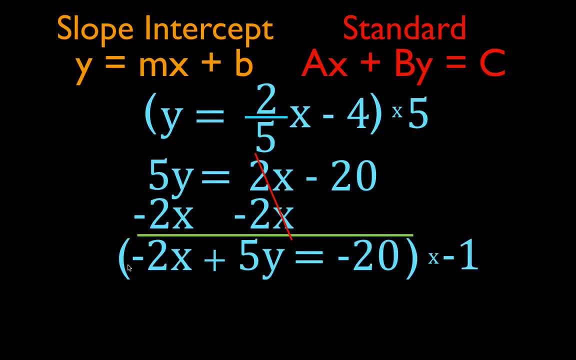 whole thing by minus 1 is we just change the sign, because a minus times a minus is a positive, a positive times a minus is a minus and a minus times a minus is a positive. So all we really do is change the sign for each term. we just get 2x plus minus 5 equals. 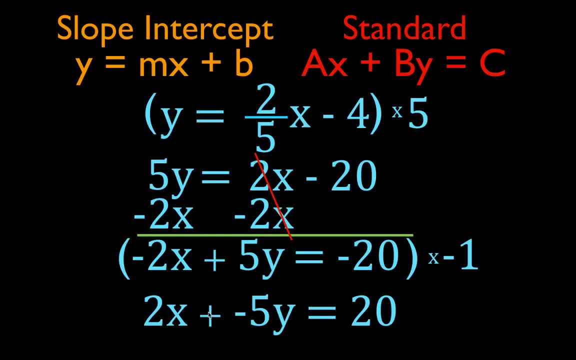 20.. Alright, And you can actually leave this plus sign out. So it'll just be 2x minus 5y equals 20.. That's how you do that one. Currently it is now in the standard form Ax plus by equals 20.. 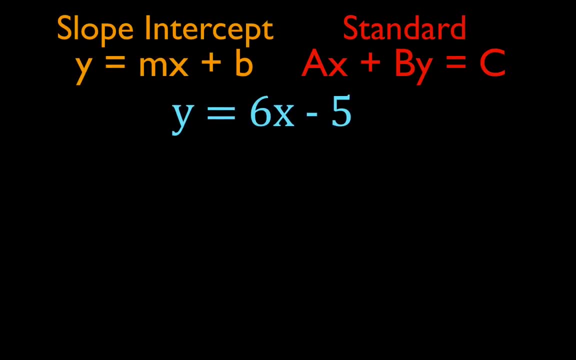 Alright, the next one Now. the first step was if the slope was a fraction, multiply by the denominator. Well, in this case the slope is not a fraction, it's a whole number. So we're just going to not do that step. We're going to skip step 1 altogether and go on to step 2.. 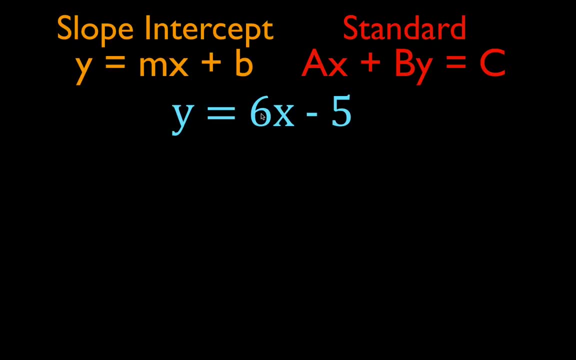 Step 2 was simply to add the opposite of the x term. This is 6x. the opposite of 6x is minus 6x. I'm going to add minus 6x to both sides. Once again, we have minus 6x. we have x and a y on like terms: minus 6 plus y. 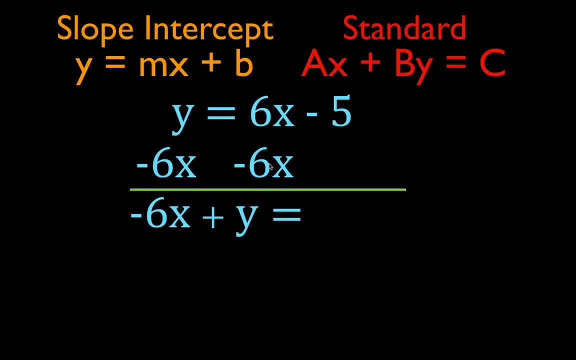 We have plus 6 and minus 6, we add those up, bring the negative side down, those cancel and you get minus y. Now, once again, we have minus 6, we've got to get rid of that minus sign. 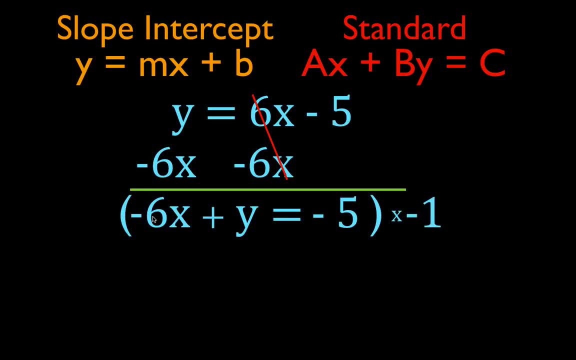 So we're going to multiply. Multiply the whole thing by minus 1.. We get 6x. change the signs basically: negative, positive, positive, negative, negative, positive. And that is that equation: 6x minus y equals 5.. 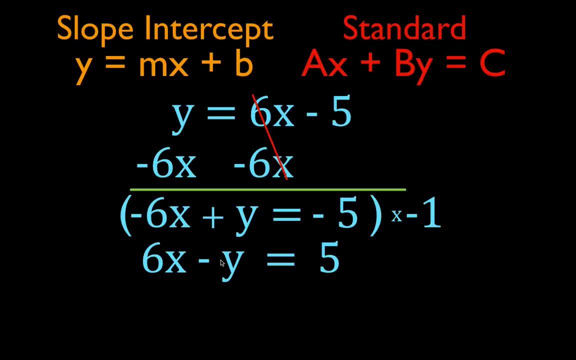 For the y term, the co-efficient b is really minus 1, but we don't write the minus 1 in The next one And the last one. Okay, y equals mx plus b. y equals mx plus b plus b. Once again, the slope is not a fraction, so we're just going to skip step one. We're. 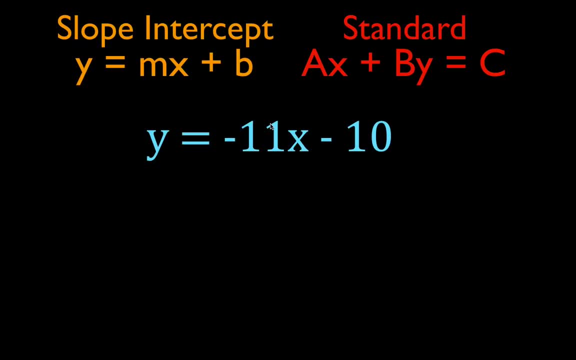 just going to go to step two, which is to add the opposite of the x term. The x term is minus 11x. add 11x to both sides. 11x plus y or y plus 11x is simply 11x plus y Then. 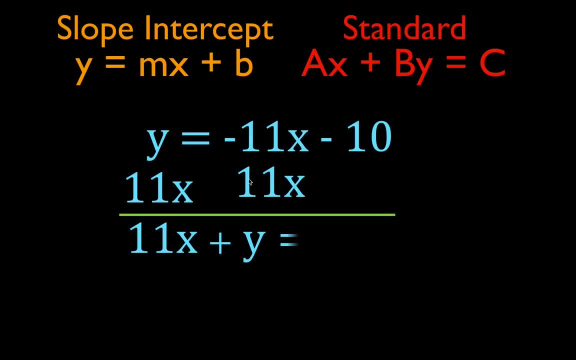 we have minus 11x. plus 11x is zero, so those cancel and you're left with minus 10.. And that is all done, right. We got ax plus by equals c. The a term is positive, We have no fractions. The b term, once again, is one. c is minus 10, and there you go. Okay, So 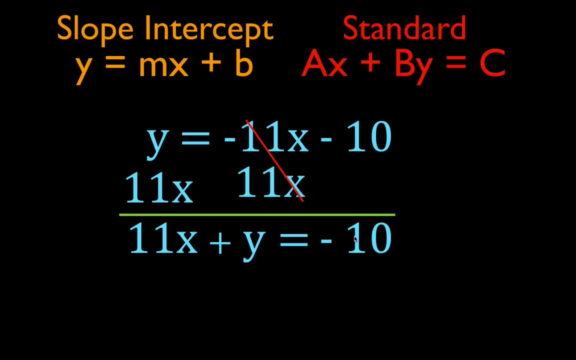 I think you can do those pretty easily. Follow those two steps. Step one: if the slope is a fraction divide by the denominator, Then step two: add the opposite of the x term to both sides and you will end up with the standard form ax. 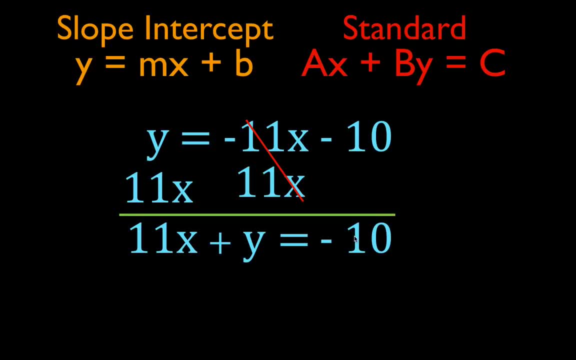 plus by equals c. Thank you very much for watching. I hope you found that helpful. If you found that helpful, you can do one or all the following three things: Subscribe to my channel, Get all my excellent chemistry, physics and math videos. 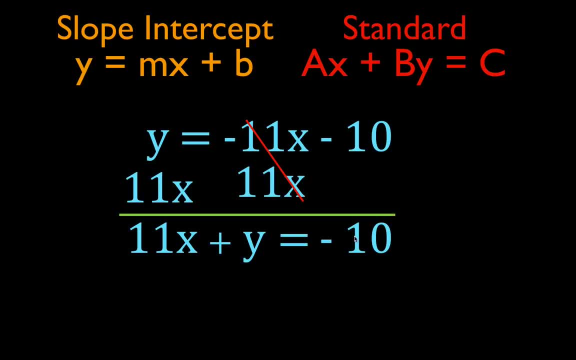 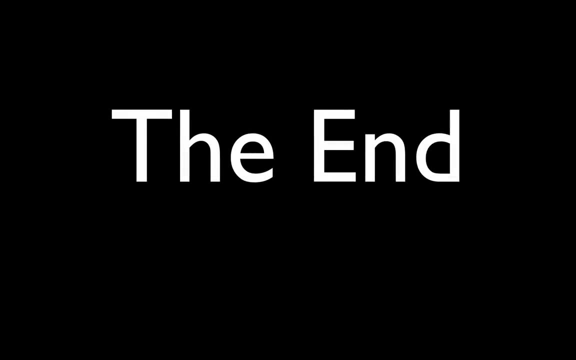 Give me a nice thumbs up for this video and leave me a nice positive comment in the comments section below. Thank you very much for watching. We will see you in the next video.